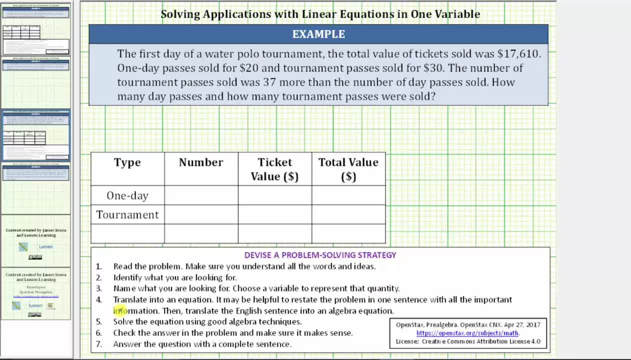 and choose a variable to represent that quantity. four: translate into an equation. five: solve the equation. six, check the answer. and finally, seven, answer the question with a complete sentence, Reading the problem. the first day of a water polo tournament. 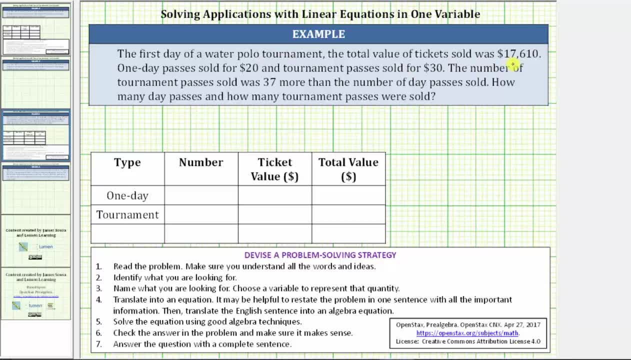 the total value of tickets sold was $17,610.. One-day passes sold for $20, and tournament passes sold for $30.. The number of tournament passes sold was 37, more than the number of day passes sold. How many day passes and how many tournament passes? 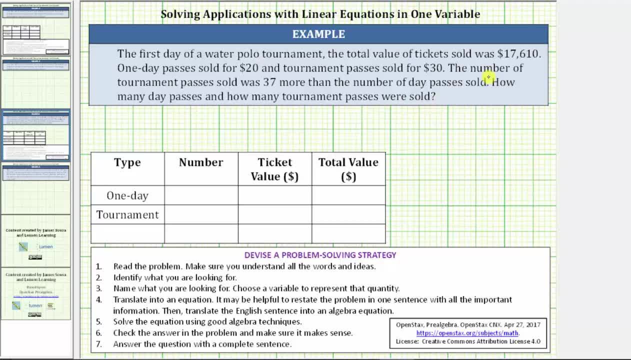 were sold. For this problem we are looking for the number of day passes and the number of tournament passes that were sold. So for this problem we do have two unknowns, but because the number of tournament passes sold was 37 more than the number of day passes sold, 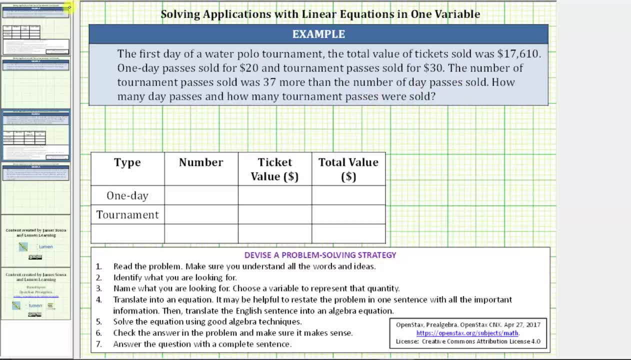 let's let the variable d represent the number of day passes sold And then, because the number of tournament passes sold was 37 more than the number of day passes sold, we can use the expression d plus 37 to represent the number of tournament passes sold. 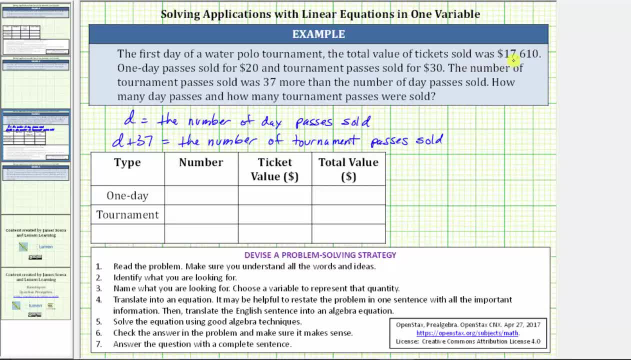 Because the total value of all the tickets sold was seventeen thousand six hundred ten dollars. let's now use this table here to come up with an expression for the total value of the one day passes and the total value of the tournament passes. So we know the number of one day passes. 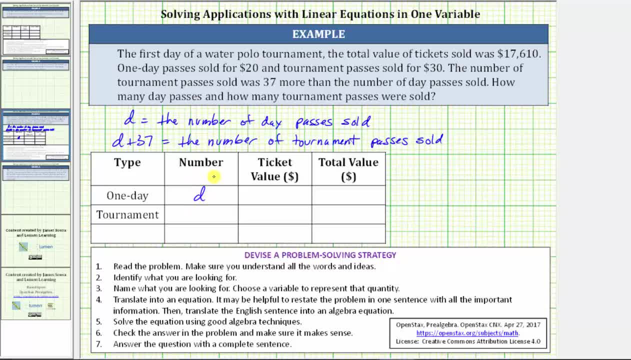 is represented by the variable d. Each one day pass costs twenty dollars, So the ticket value of each one day pass is twenty dollars, which means the total value of all of the one day passes is twenty dollars times d or twenty d. And now for the tournament passes, the number of tournament. 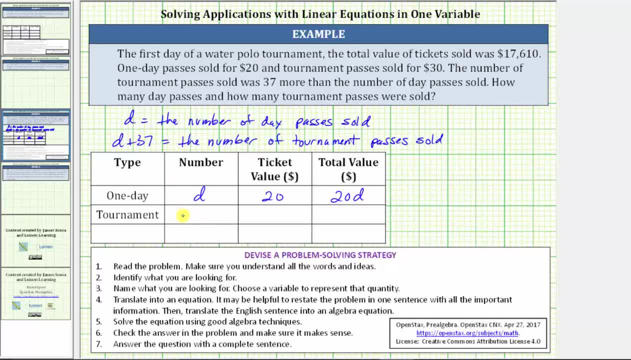 passes is represented by the expression d plus 37. The ticket value of each tournament pass is thirty dollars, or twenty to left equal zero, Which means the total value of all of the tournament passes is thirty dollars times the quantity d plus 37, or just thirty times the quantity d plus 37. And we know the value of. 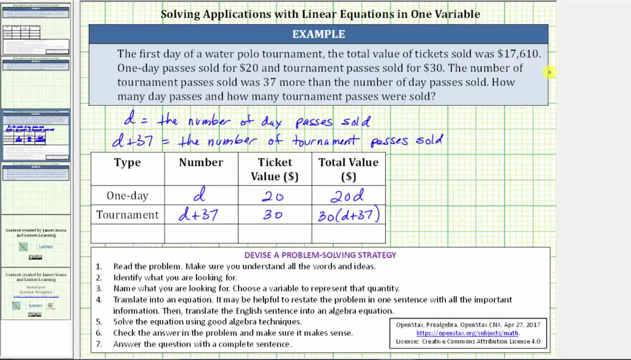 all the tickets sold is seventeen thousand six hundred ten dollars, which we'll record here And now we have all the information we need to complete step four, which is to translate the information into an equation Using this, this last column, the value of the one-day passes. 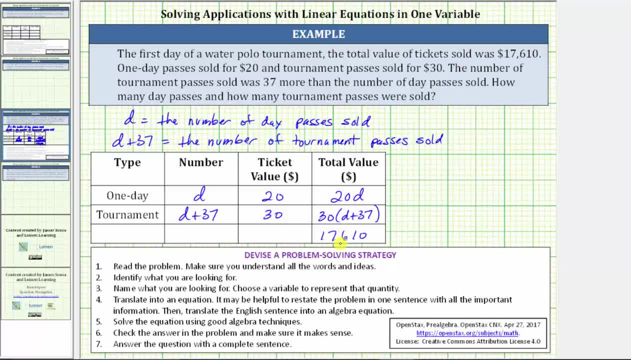 plus the value of the term that passes must equal $17,610, which gives us the equation: 20d plus 30 times the quantity d plus 37 equals 17,610.. The next step is step five, to solve the equation. Then step six is check the answer. 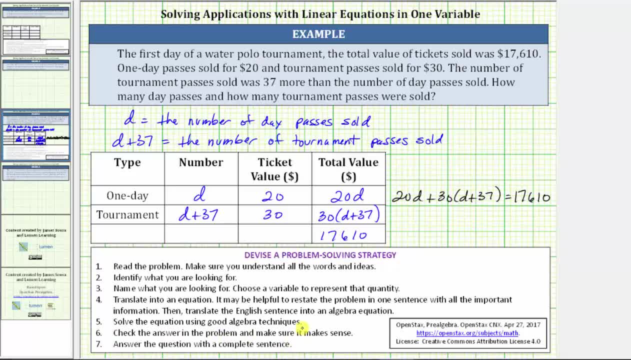 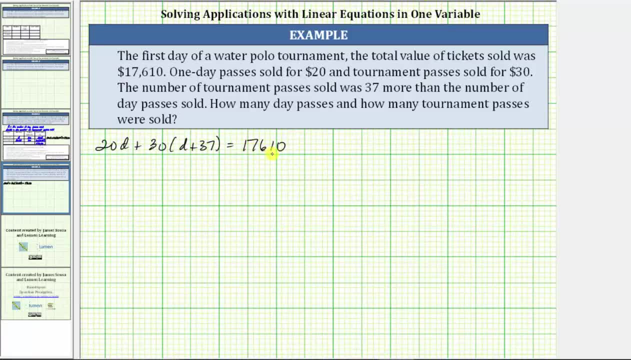 Finally, step seven, answer the question with a complete sentence. Let's solve this equation on the next slide. The first step is to simplify both sides of the equation. The right side does not simplify, but the left side does. We simplify the left side by clearing the parentheses. 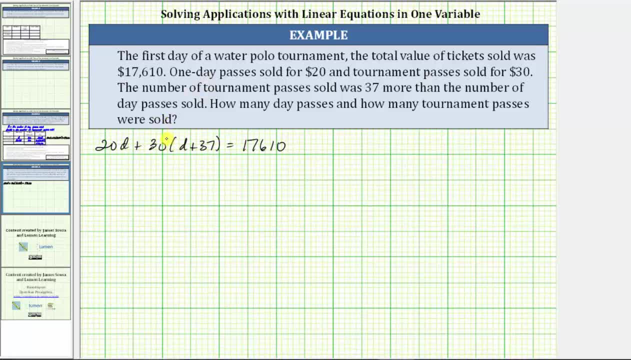 and combining like terms, which means the next step is to distribute 30. This gives us 20d plus 30 times d is 30d plus 30 times 37 is 1,000. That's 1,110.. Still simplifying the left side, we combine like terms: 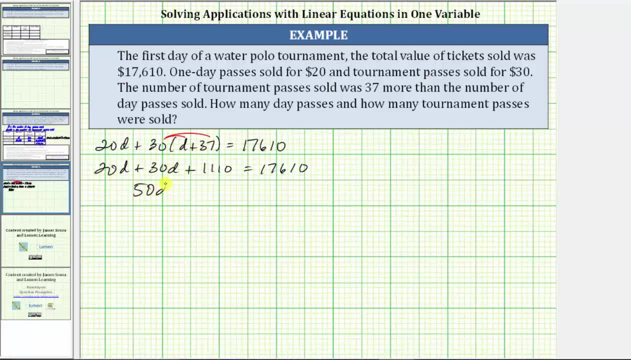 20d plus 30d is 50d. We have 50d plus 1,110 equals 17,610.. The next step is to add or subtract, to isolate the variable term and combine the constants. on the other side, To isolate 50d we need to undo plus 1,110. 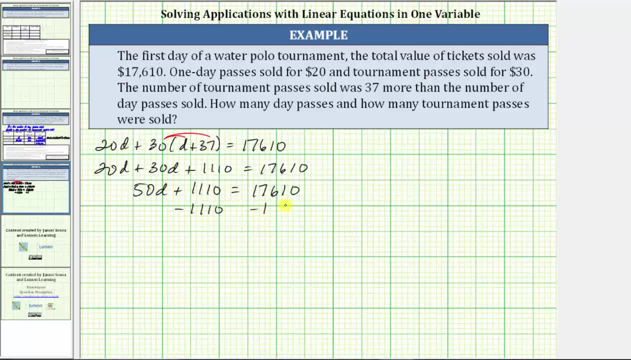 by subtracting 1,110 on both sides of the equation. Simplifying 1,110 minus 1,110 is zero. The left side is now 50d equals. on the right side, 17,610 minus 1,110 is 16,500. 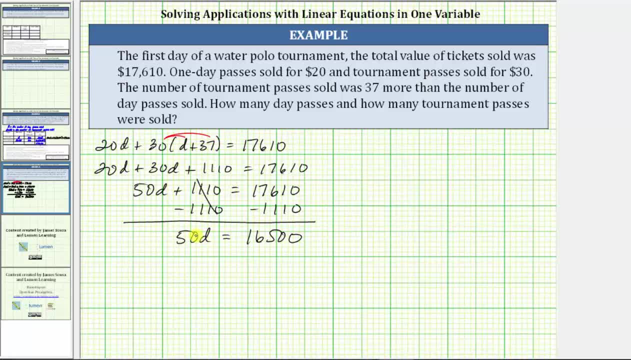 Now that we've isolated the variable term, the next step is to multiply or divide. To isolate the variable and solve for d, Because 50d means 50 times d. to undo the multiplication and solve for d, we divide both sides by 50.. 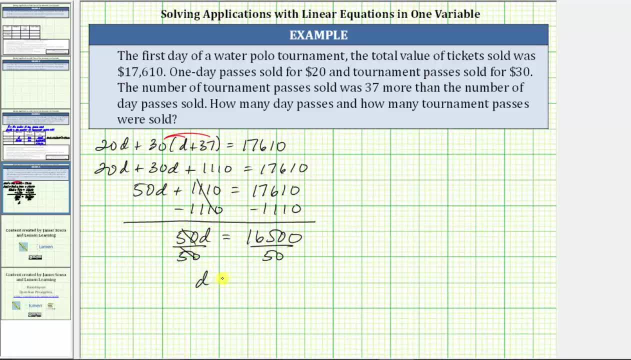 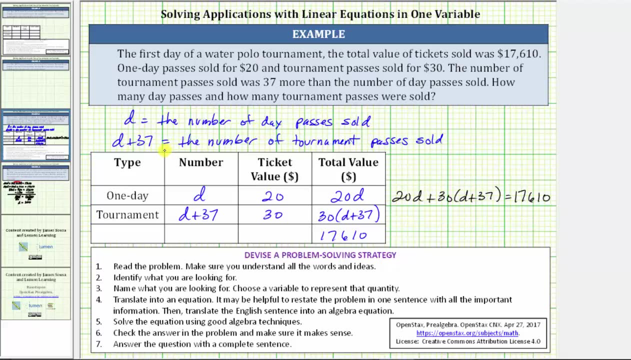 Simplifying: 50 divided by 50 is one. One times d is d. We have: d equals 16,500, divided by 50 equals 330.. And remember, d is the number of day passes sold, and d plus 37 equals 1,000. 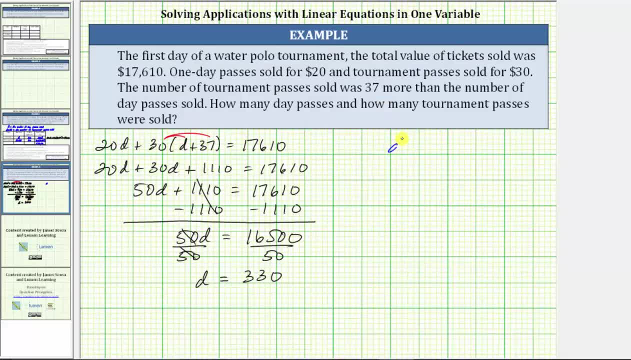 1,000 is the number of tournament passes sold. So we know d equals 330, and d plus 37 is equal to 330 plus 37,, which equals 367.. Before we write the answer as a complete sentence, let's check this answer by using these values. 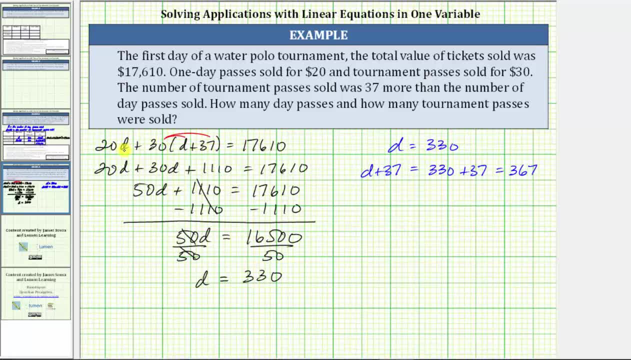 in the equation here, where we substitute 330 for d and 367 for d plus 37, which gives us 20, times 330 plus 30, times d plus 37 is 367, and this must equal 17,610.. 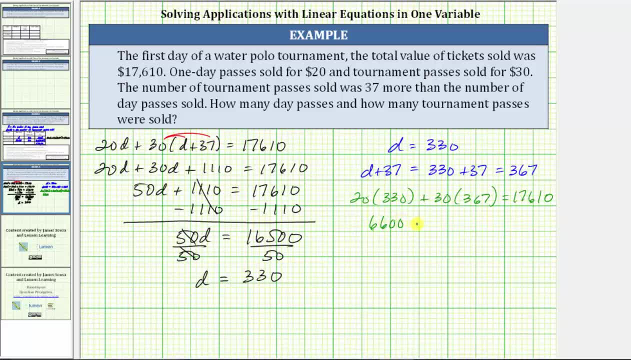 20 times 330 is 6,600, plus 30 times 367 is 11,010.. 6,600 plus 11,010 is 17,610.. 6,600 plus 11,010 is 17,600.. 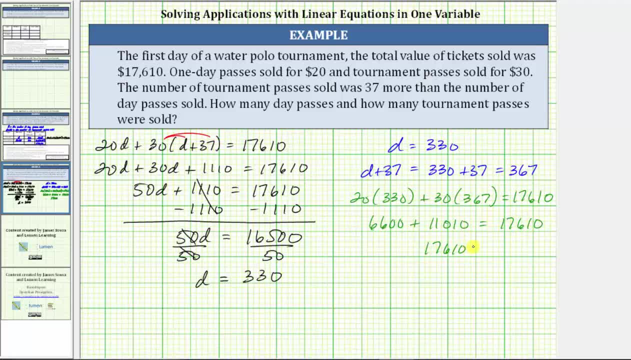 plus 17,610.. plus 17,600.. plus 17,610.. ten. So, because we have a true statement here, this verifies our answer is correct. So, as a complete sentence: 330 day passes were sold. 367 tournament passes were sold. 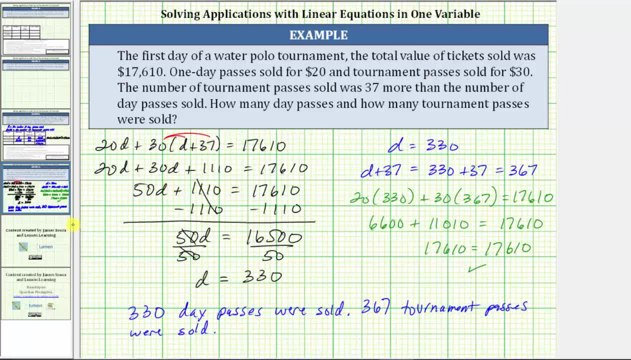 Or I should say two complete sentences. I hope you found this helpful. 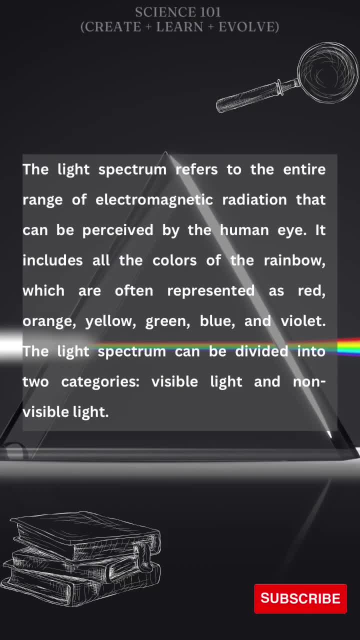 Science, you thought you knew The light spectrum. The light spectrum refers to the entire range of electromagnetic radiation that can be perceived by the human eye. It includes all the colors of the rainbow, which are often represented as red, orange, yellow, green, blue and violet. The light spectrum can be divided into two categories: visible light and non-visible light.